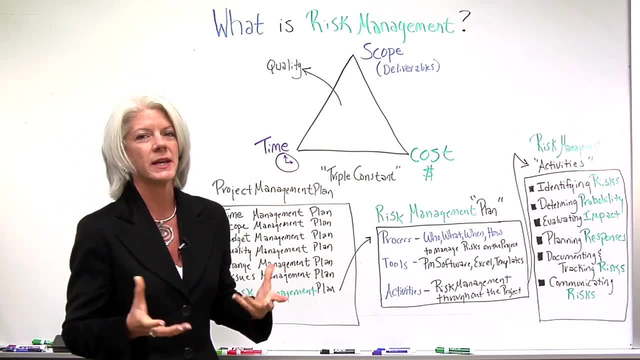 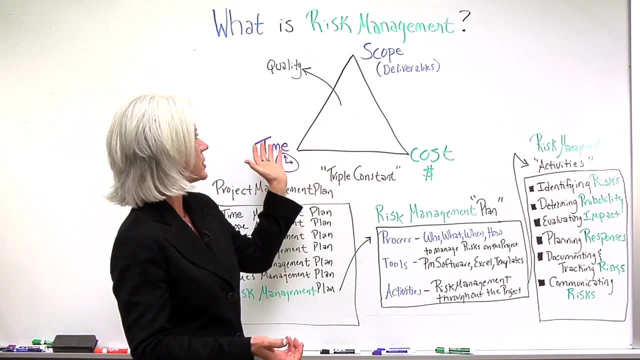 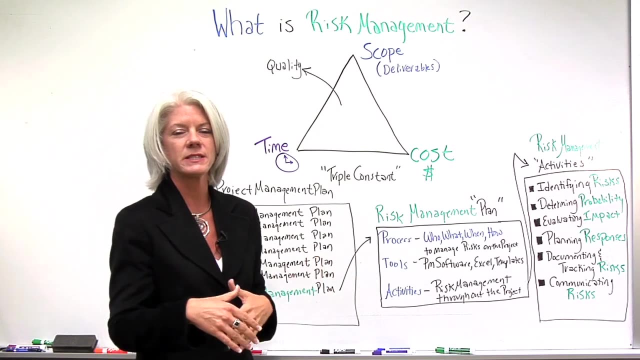 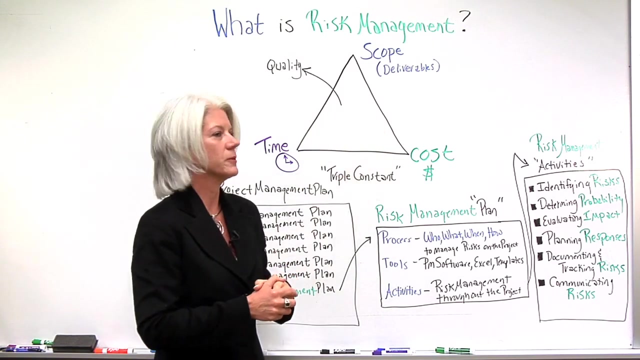 which again is referenced as the triple constraint. So throughout the project, different events occur. maybe things happening with scope or cost, or changes in the schedule or quality occur that could introduce risk, or vice versa. Different events can occur throughout the project that also can impact these components as well. 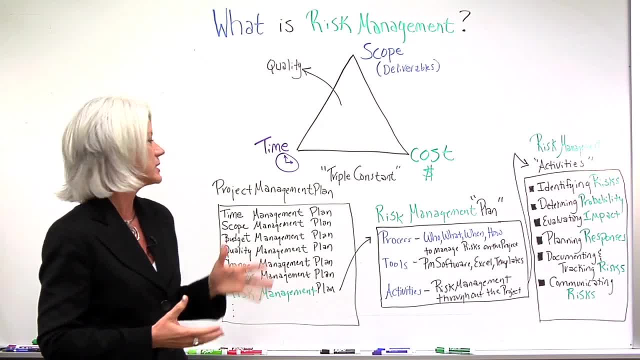 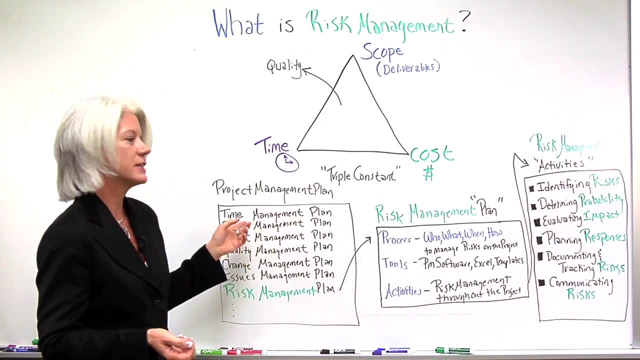 So, basically from a high level. when we talk about the project management plan, we know that the project management plan also has other plans, subplans in it as well, like the time management plan, scope management, budget, quality, the change management plan and issues. 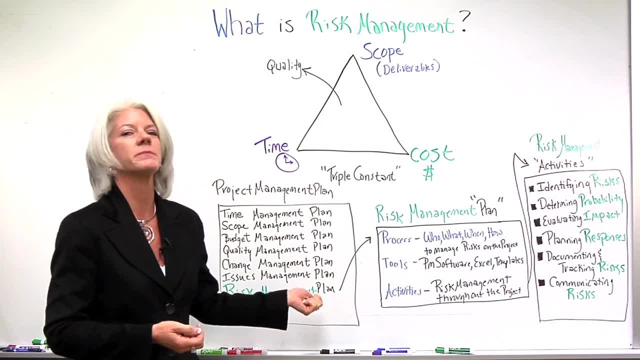 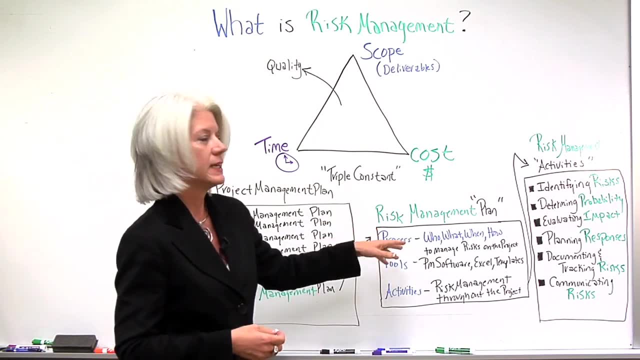 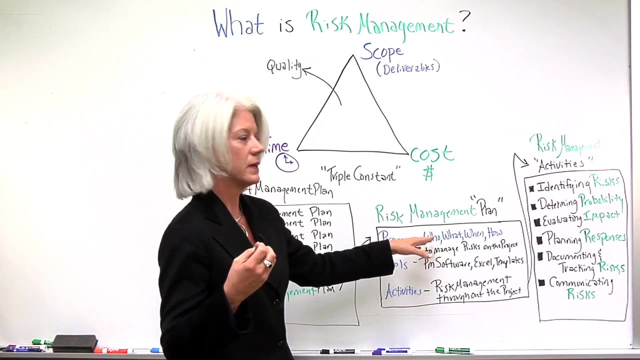 But also the risk management plan is a subset or subplan of the project management plan. So basically, what is entailed in the risk management plan is the process. We want to know, who needs to know, who can interject risk into the project. 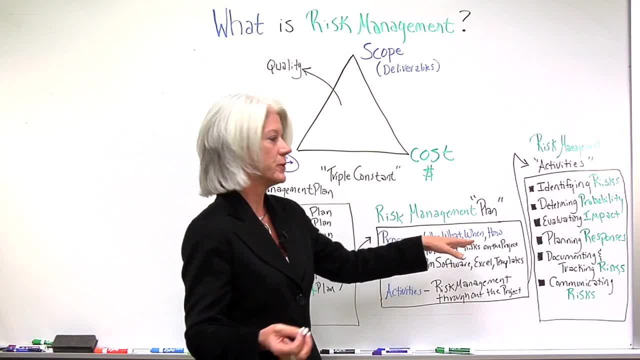 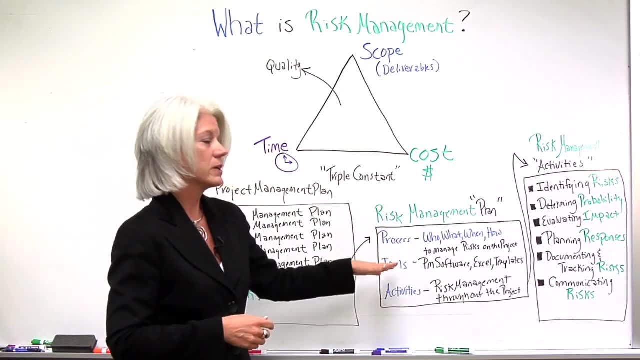 what's the process, when do we do it, how do we do it? So, basically, the who, what, when, how to manage risk on the project. We also look at tools. We identify what tool set we're going to use. 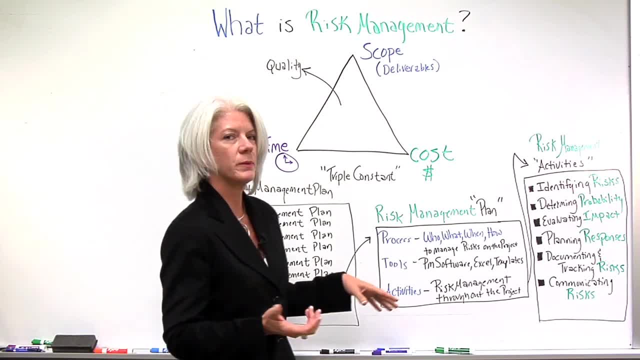 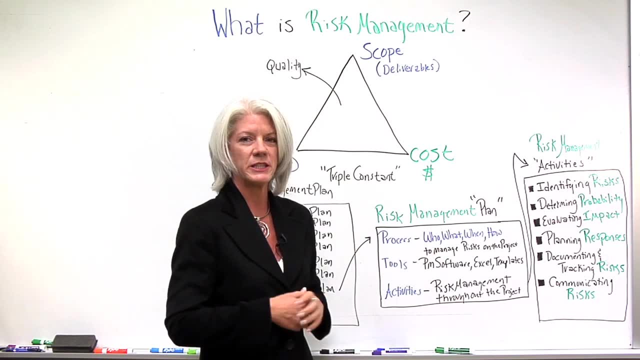 So everyone on the project who needs to know or involved will know what tools to use. So we identify. we're going to use project management software Now. a lot of the project management software available today are great with helping to assist in identifying and managing the risk. 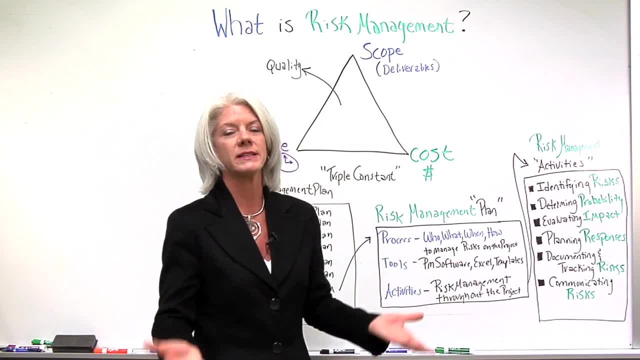 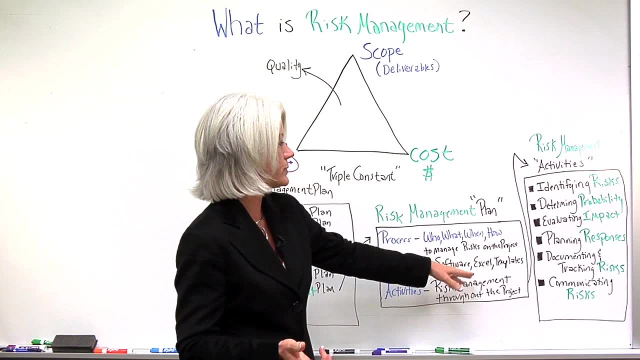 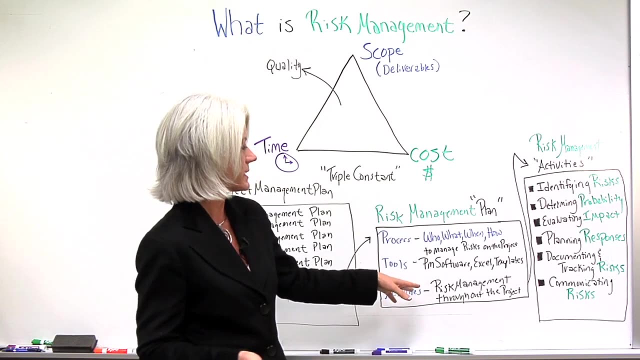 A lot of people still use Excel, So they have Excel where they have the logs and the registers and any kind of templates, The templates we may use to identify and evaluate the risk. So the activities included in the project management plan are identified here. 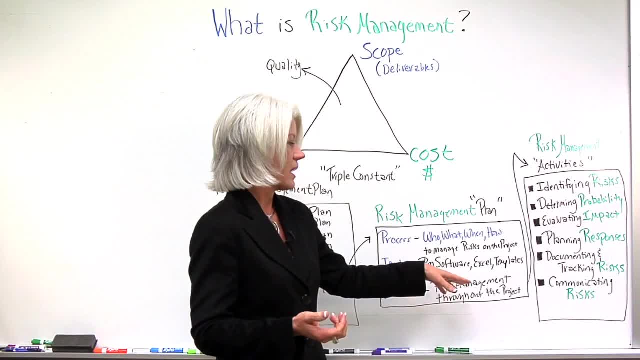 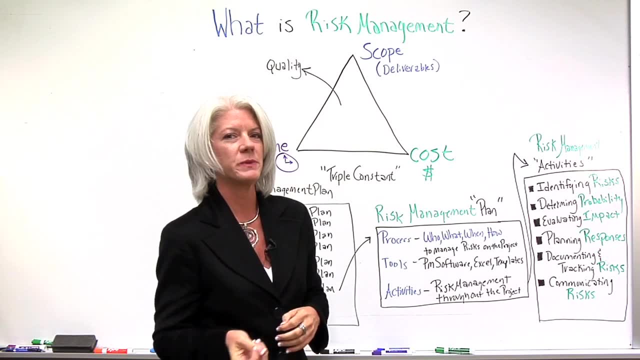 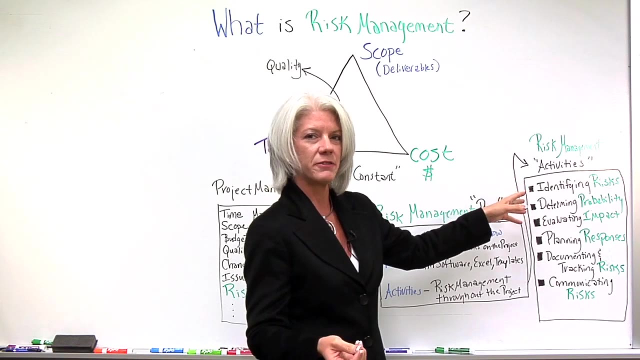 But basically it's all the activities that we use to manage risk throughout the entire project. So what are some of those activities? So risk management, the risk management activities, are about the activities to identify the risk, Like how do we go about identifying what documents? 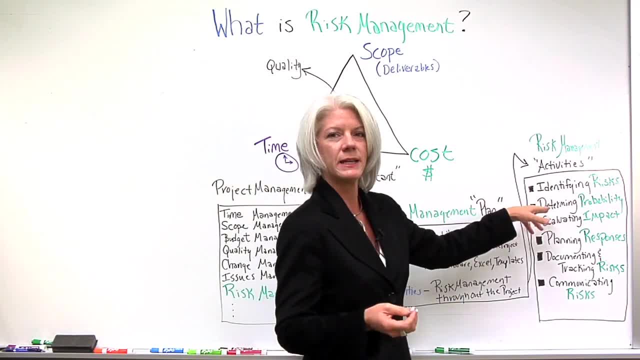 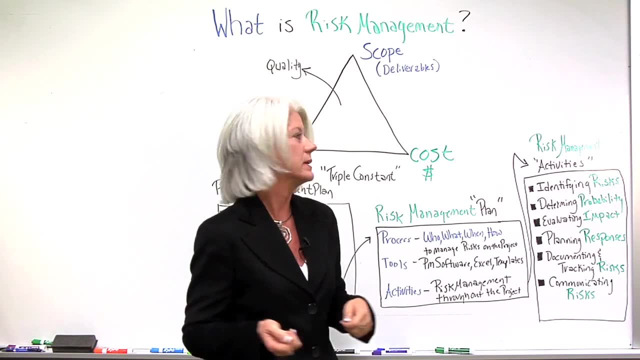 or what things do we look at determining When we do identify those risks. we want to determine what's the probability, What's the probability that this will happen, and evaluating the impact. If it does happen to occur, what would be the impact to the project?